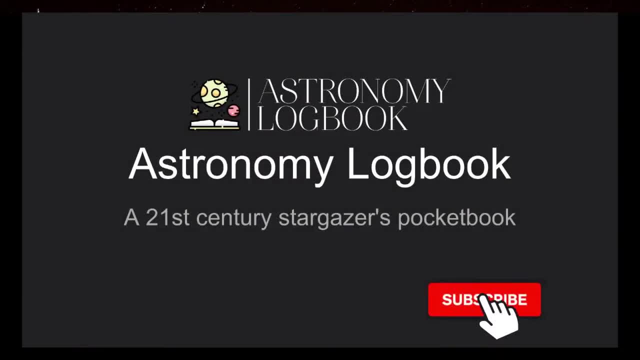 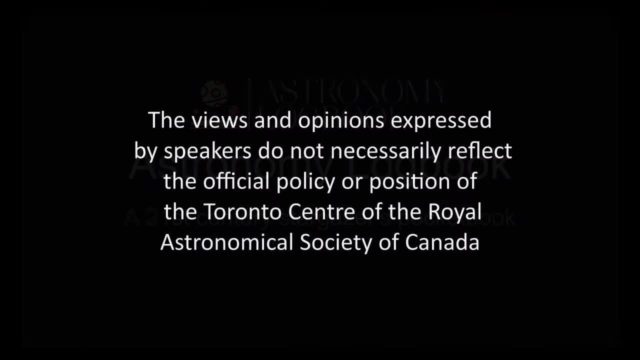 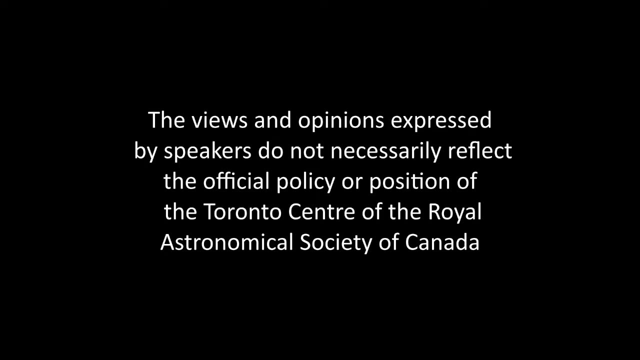 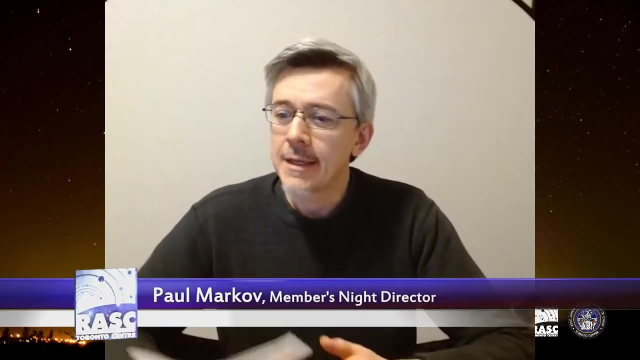 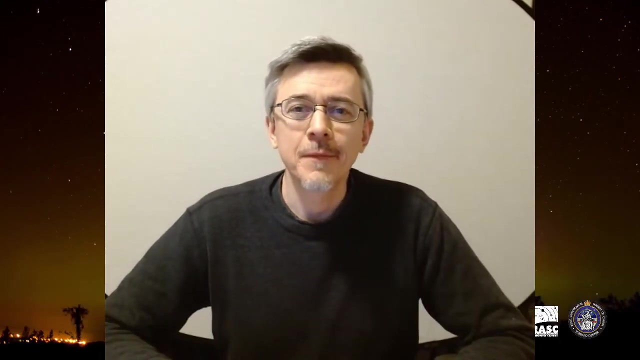 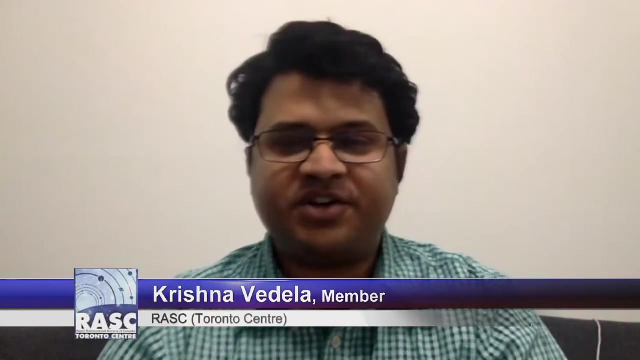 Let's move on to our next speaker, and that's Krishna Videla, and he'll talk to us about the observing logbook. Go ahead, Krishna. Hello everyone, I'm Krishna Videla, from Toronto. I want to talk to you about an astronomy logbook. 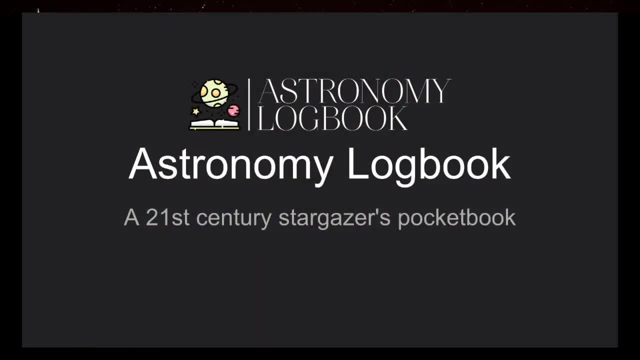 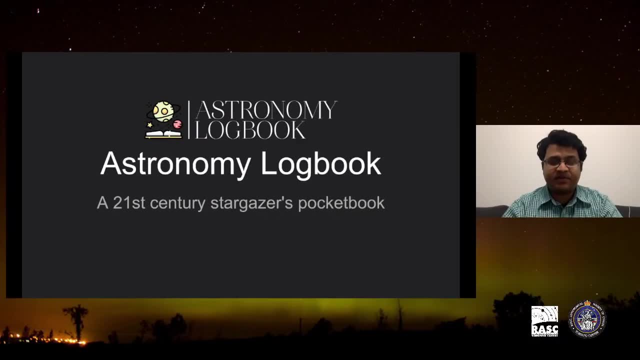 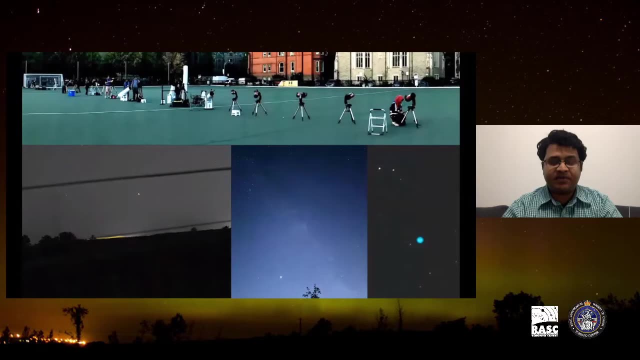 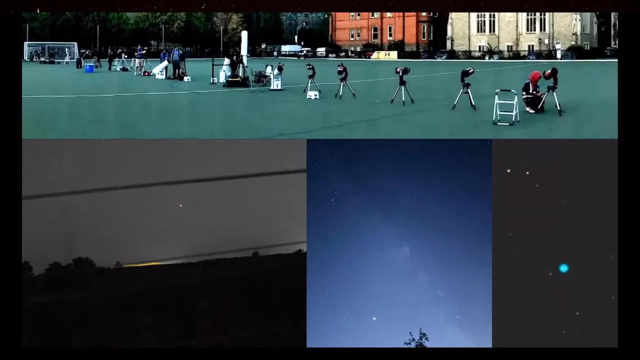 that I thought was quite helpful for me to record my observations whenever I do start. We all know we all started observing skies at some point in our life. Usually it started with watching the night sky, just sitting there with our family, friends, and slowly we start. 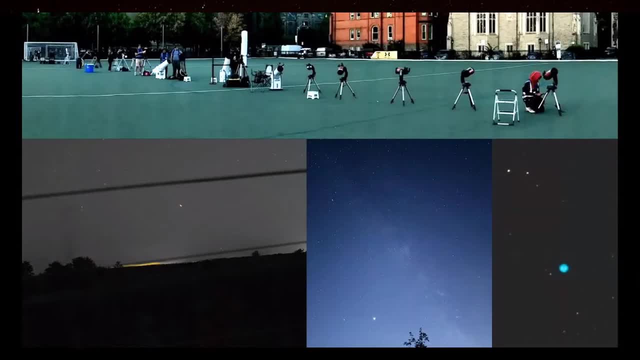 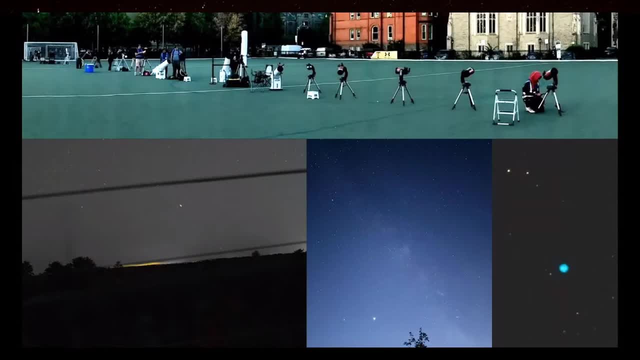 see something quite different. You might see something quite different. You might see something interesting up in the sky. So, for example, to the left-hand side, bottom left of the screen. you see what I thought I was picturing: an aurora from right here in Toronto, in fact. 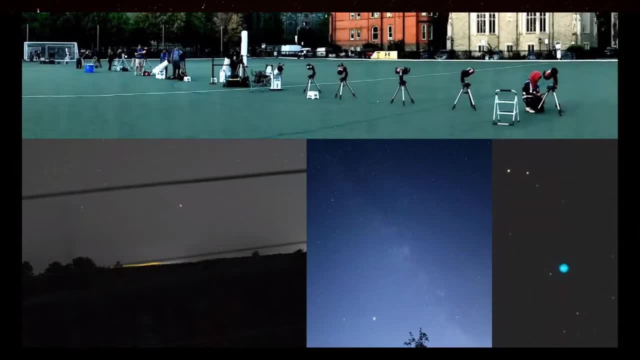 outskirts of Toronto. Whether it is true or not, I wouldn't be able to know until I go back and check the records. if that is indeed the fact, Not only that, sometimes you might be observing the sky, but you might be seeing a picture of a celestial object To the right-hand side, here is a 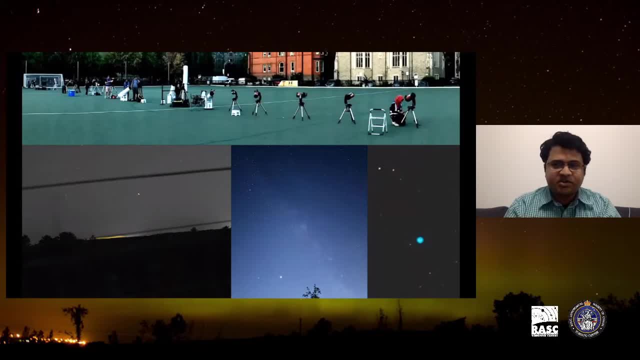 blue snowball nebula. It is an NGC object, quite faint, easy to detect from an 8-inch telescope, or at least that is what I heard. So I spent about four hours trying to find that object And unless I know when I did that, what time I recorded, what was the sky conditions? what were the sky conditions? 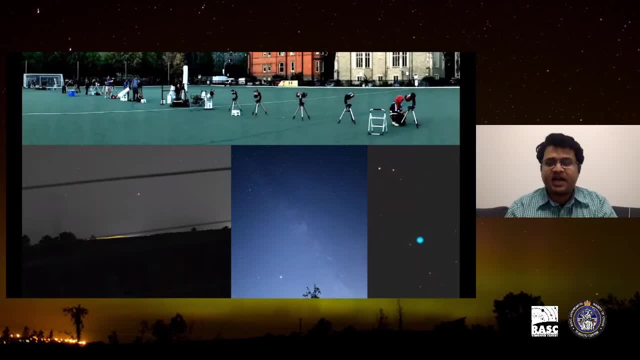 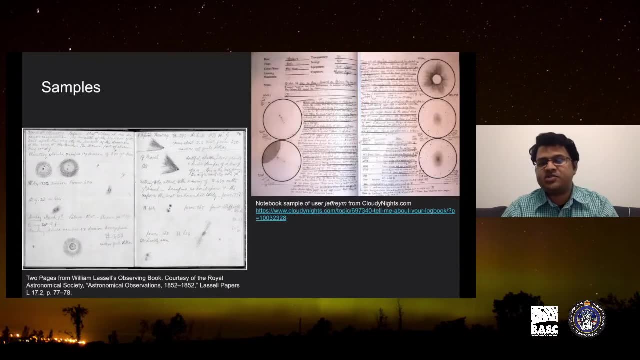 like I wouldn't be able to go back and recreate the same situation and say I was spending four hours looking for it again, And that leads us to recording these observations. These are some examples of how people others have recorded what they observed, going back to 1800s And, in fact. 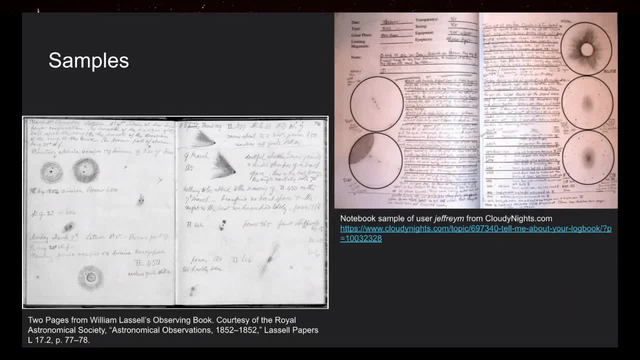 these observations, these recordings and these notes that they made at the time have proven quite useful, not only to them but also to other people, But for later researchers who look back and see what was the magnitude of the star at the time, what was the 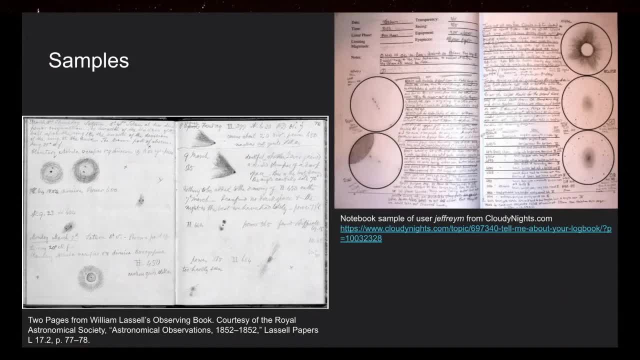 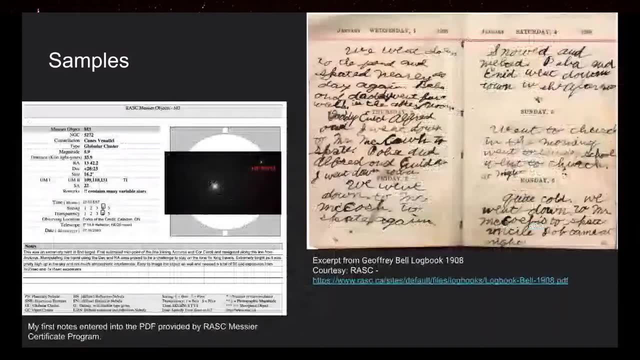 shape of that object at the time? did it change from then to now? and so on and so forth? Now the handwriting can be quite legible, like the one here on the left-hand side, or it can be completely legible, However it is. 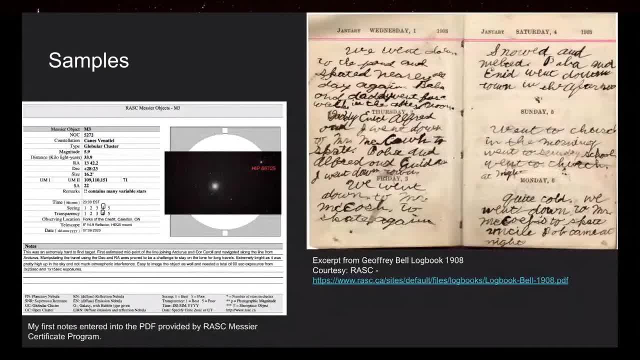 an observation nonetheless, And RASC has provided good PDF files to record such observations, to make such recordings in a very concise and in an organized fashion. So the left-hand side is a snippet from RASC's Messier Object Certificate Program where we can record what the object is. at what time did we record some of these details? 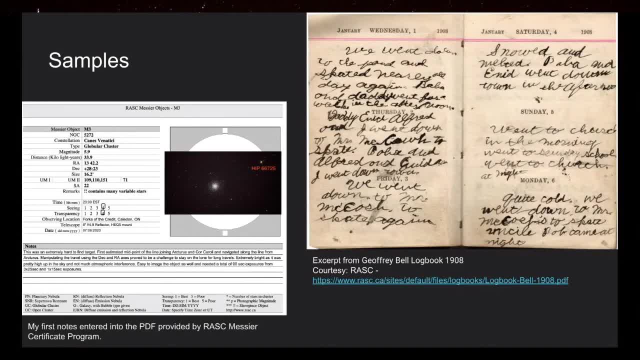 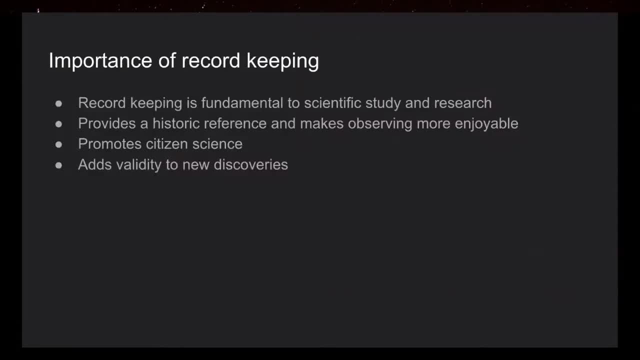 And it also allows you to make some additional notes that you can add for the observations at that time, And it is very important for us to do so because it promotes citizen science. Like I said, it allows us to come up with new discoveries. 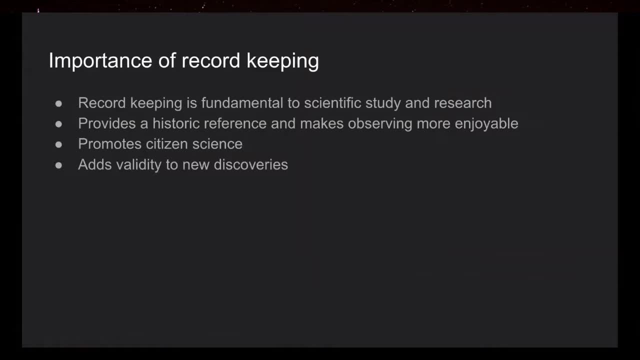 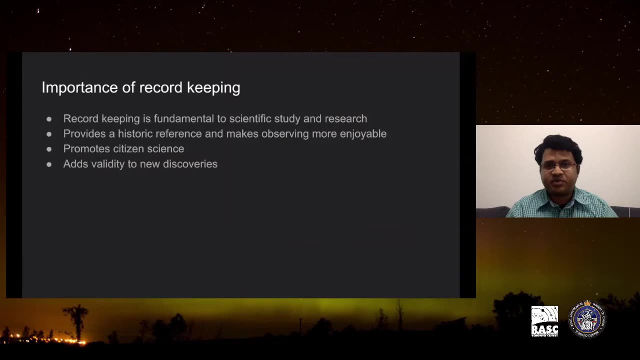 What we saw before. there might be a star that you have not seen, but today it doesn't appear anymore, which could mean that probably it's a supernova explosion or something like that. So it is very important for us to do the record keeping of these observations, whether we do it casually. 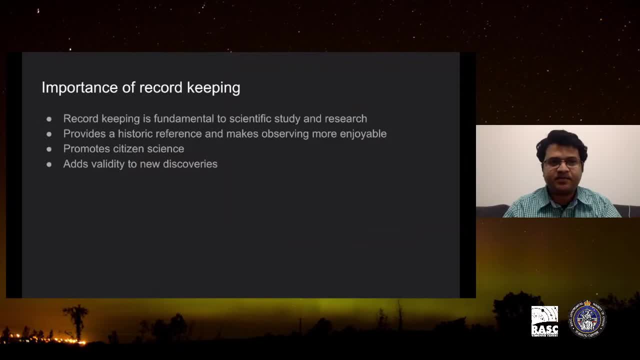 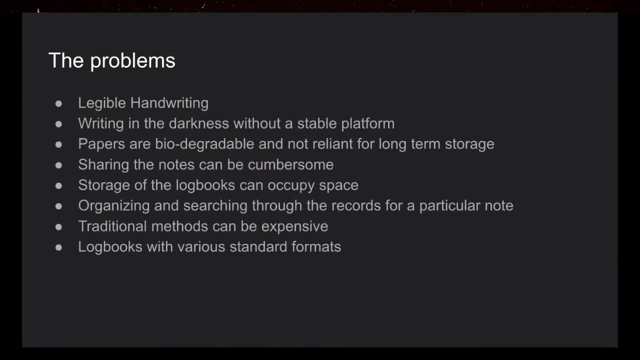 Or whether we do it for scientific purposes. When we try to do these recordings in a dark sky situation, there are plenty of problems that we face. First and foremost, it is very difficult to write on a piece of paper or in a notebook when we do not have a table with us. 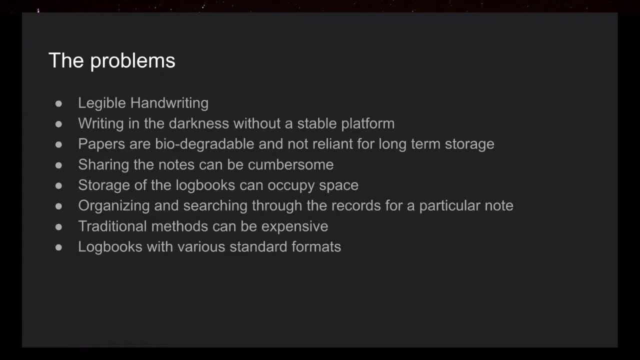 And carrying a table along with the telescope, along with your observation equipment and all of that. it could be quite a daunting task. The papers, if we write them on our… on our, if we write them, if you write, if we make our notes on on a piece of paper, it it doesn't. 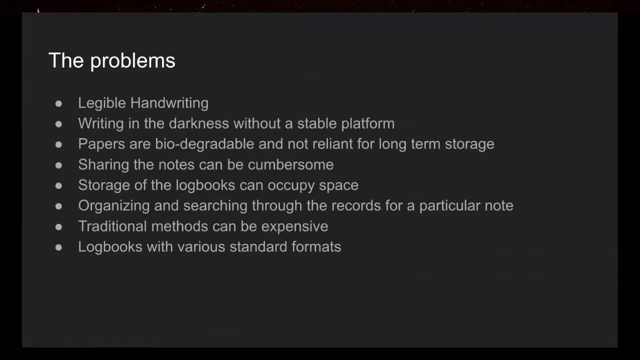 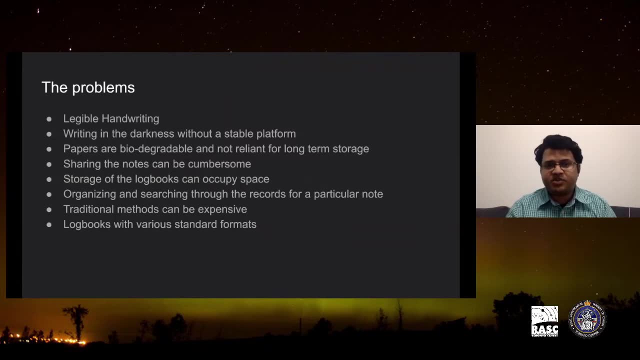 stay. it doesn't stay for too long. it can. it can get destroyed if water spills on it or if you put a coffee on it and we cannot even search through those notes to. in order to go through and refer to a note that i made back in um back in 2018, i would have to go through a notebook dated 2018. 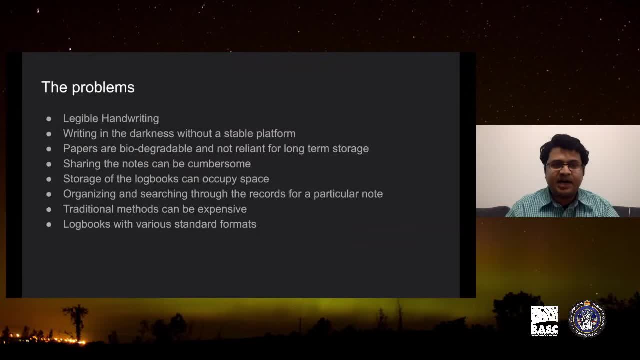 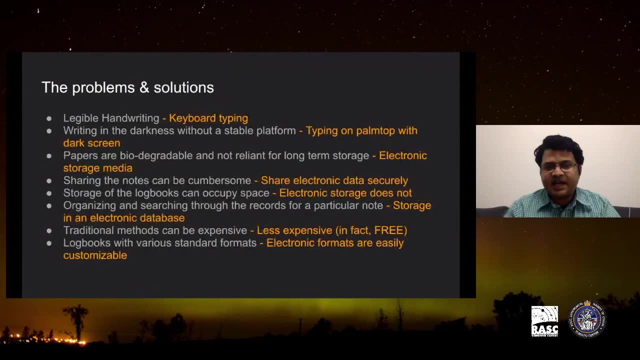 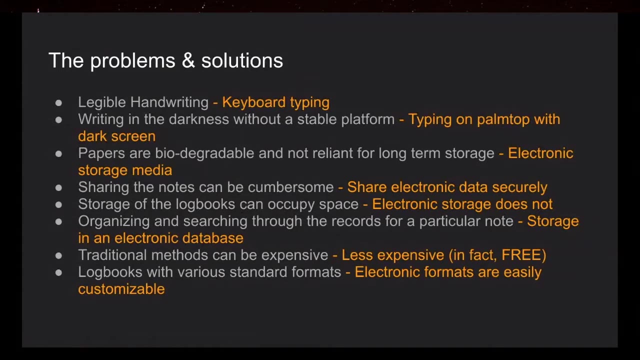 rumble through the pages and then find out which one that is um so it, but today we are living in the 21st century- can we come up with a solution for all these problems? and that's exactly what what i thought to myself when covet hit and um, and we were in the lockdown couldn't go out anymore. 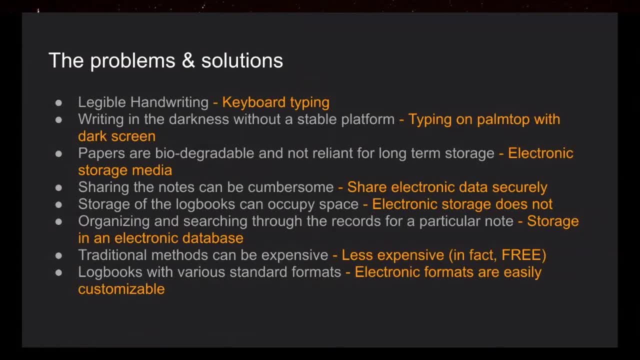 so, okay, let's look at these problems and the solutions that we can address one by one. legible handwriting. we can replace it with keyboard typing. if we, if we are in a dark, dark area and we don't have a piece of paper, can we use our smartphones? 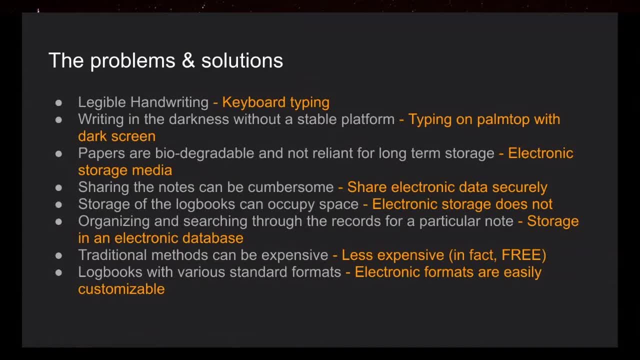 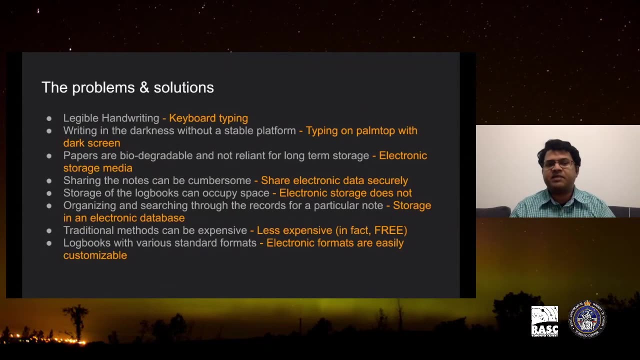 or a or a tablet screen to do that. yes, um. similarly, we can um. if we, if we are able to store these information in in electronic format, like an excel spreadsheet or some date, some kind of a database, then we can go and search through them with a single query, or um in a more electronics. 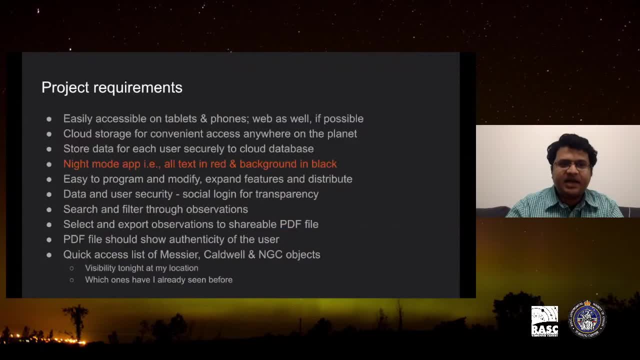 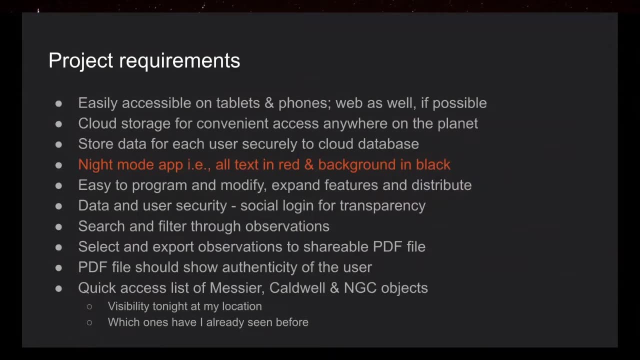 way in a much more rapid fashion, and that was that gave me the, that gave me the requirements of what i needed to do. um, because this was, this was this was the problem that i was facing myself. every night, i would go and observe: i'm trying to get in order to work for my messiah certificate. 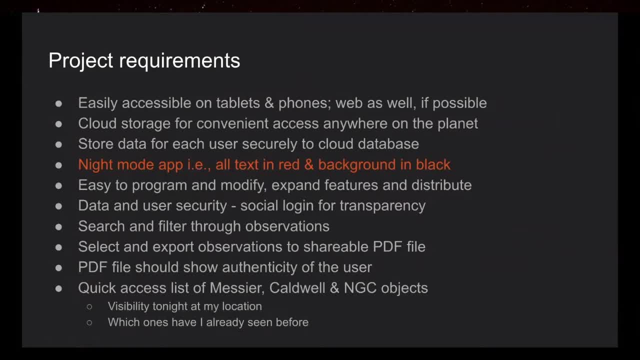 i would, um, i would take a couple of piece of paper or note. in fact, i have a notebook with the red light, try to write down my notes in there, come back home, and then i would look at the pdf file. all of this was quite, um, quite inundating and i thought you. 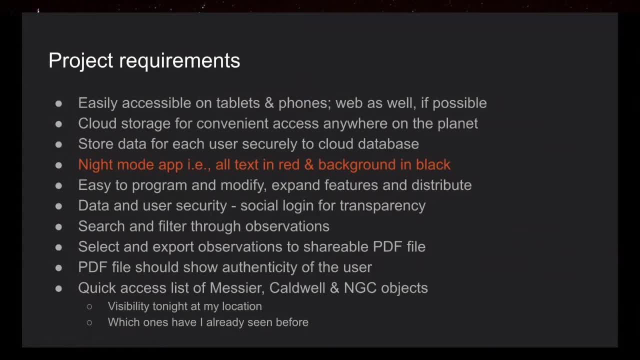 know we could do it much better, so i needed some. i needed to come up with some solution that would work on tablets, phones, um, in fact, even web. i do not need a particular type of device. if if i can store all my data in in a web-based platform, then i would. i can access it from anywhere. i do not. 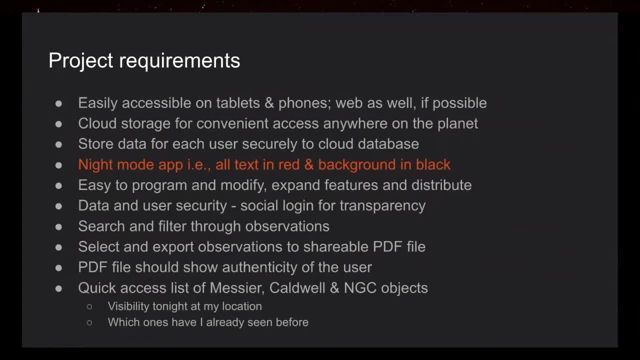 have to restrict myself uh to observing within, within my data, and i can do that by using a lot of data. i can access it from anywhere. i do not have to restrict myself uh to observing within, within my uh, in the vicinity of my home, uh with where wi-fi is available, or um go far when i travel outside. 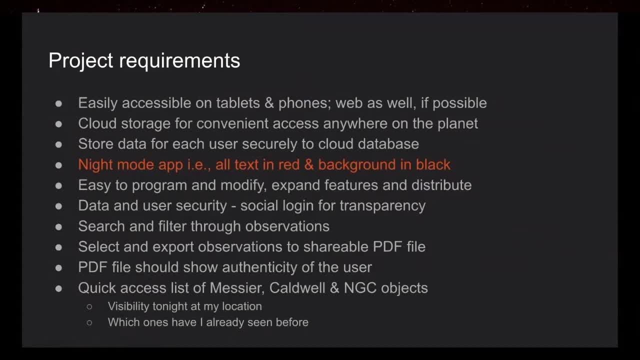 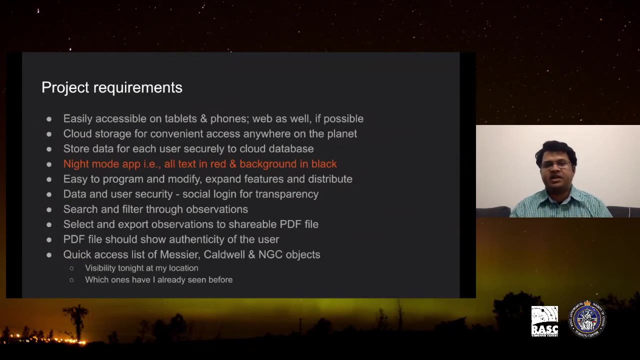 of canada. in fact, i would. i can, i can still access it and update information in there? um, because it has to work in a dark um, in a dark environment, i need to make it up in a in a, uh, in a night mode. that is all. the text would be in red and the background is black, so it doesn't affect my. 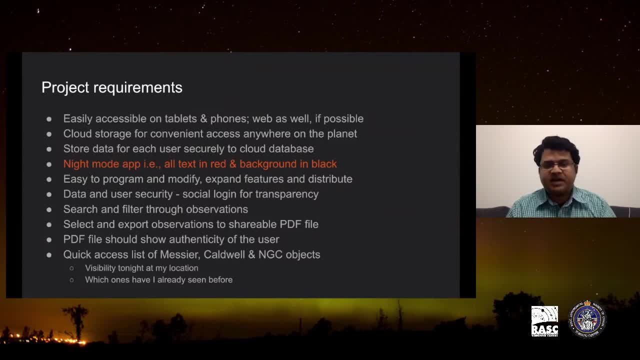 night vision the the data. whenever i store it in the cloud i, i want to keep it secure and nobody should get access to it. today i'm storing just my um observing information, but tomorrow i might store something else, so i need to make it future proof. i need to have an ability to go through and search through the observations, filter out. 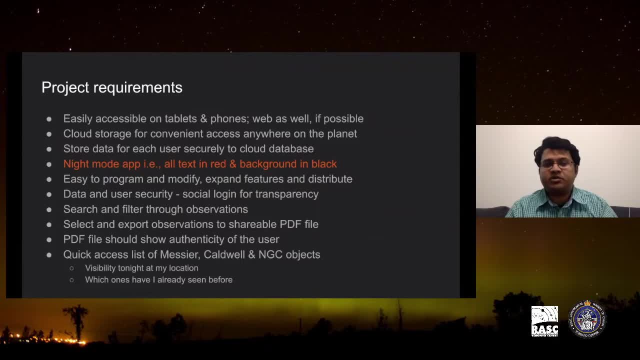 and and select which ones i want to. i want to look at again. for example, give me all the instances of observing the crab nebula like, like one of the previous speakers mentioned, it would keep changing its shape over a period of time. so if i observe it today, i want to make sure, if i observe 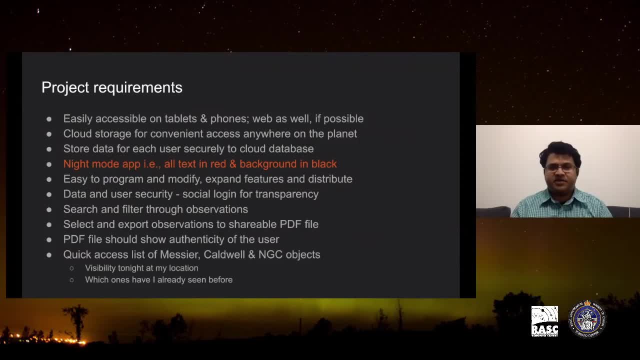 it again, 10 years later. has there been any difference? did it go? did it change in its brightness, or is it still the same? or, in fact, has it gone bigger in the? um, in the conditions of my field of vision? um, then, in order to get my certificate, 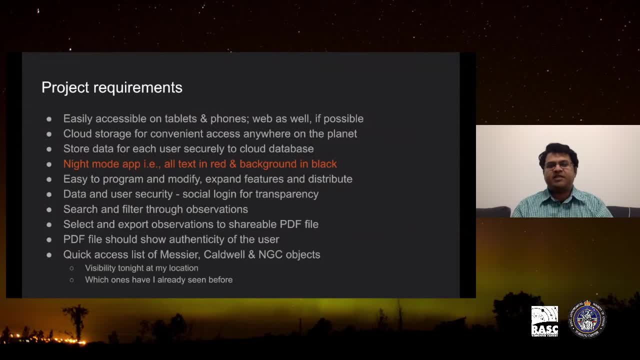 i want to, at the end, be able to convert all that information, all those observing sessions, into a convenient pdf file that i can give to rsc and hopefully they would accept it and say: yes, you can, you, uh, you get the certificate, so i should get that. um, similarly, i want to be. 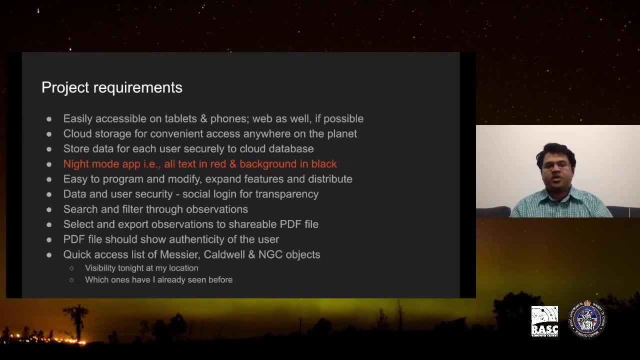 able to know, if i go out tonight, what are the messy objects, what are the objects that i would that i would be able to see immediately. i do not want to go to another app and figure out, okay, in this location, in this given period of time, which of these messy objects are visible. 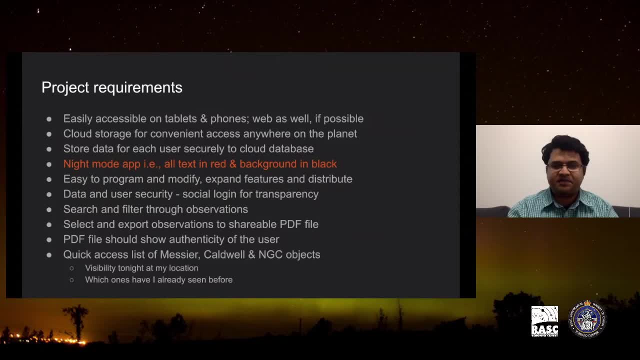 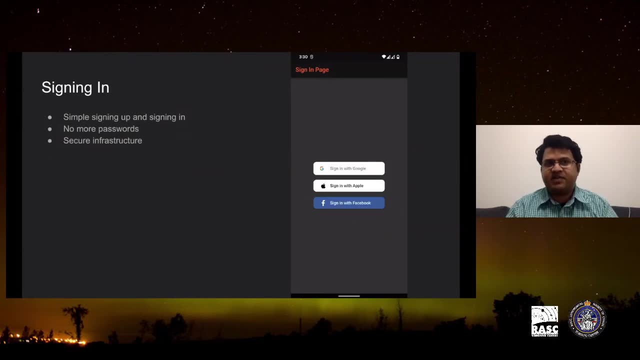 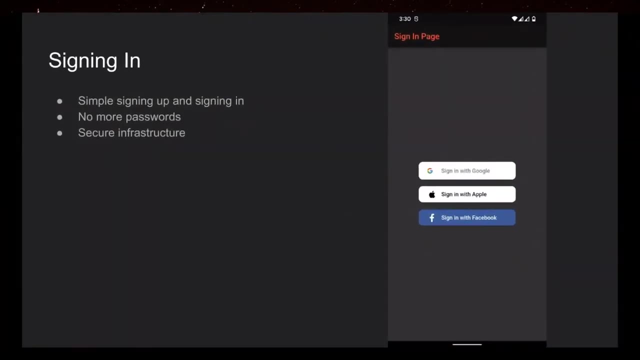 so, as a convenience, i wanted to have that ability to show up as well. that led me to build this app, called as that i that i call astronomy logbook. it starts with a simple sign in page which and it gives you the ability to sign in using google. 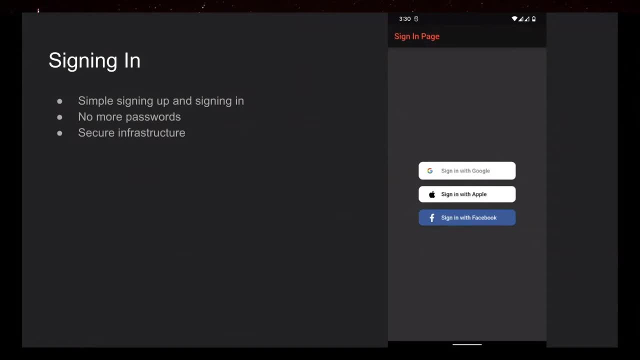 apple and facebook. so i don't want, i don't, i don't want myself or anybody else using it to worry about passwords, to worry about a new login information, and whatever existing login authentication mechanisms you have, you can continue to use it. just one last thing to remember, one more simple step. 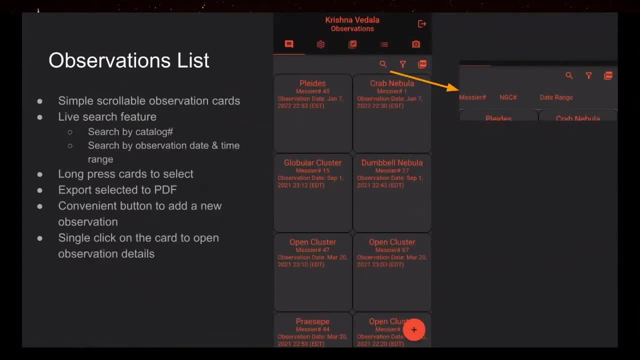 and this is the once. once, once a person logs in, you are presented with your list of observations that you have done so far. um, so, as you can see, it's a. it's a scrolling list of every observation, and each observation is presented to you as a tile. um, on the top is 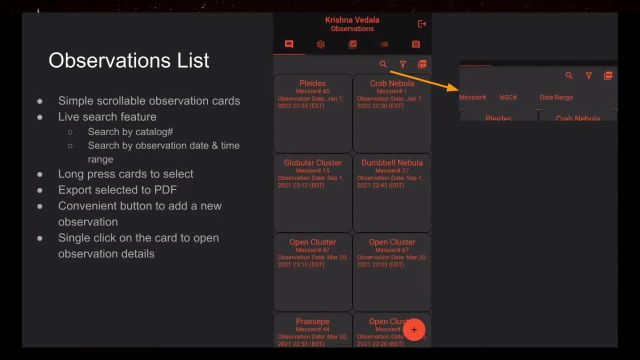 your title if if you have a messy number that mentioned in it, you can have that. that is presented over there and they're all organized in the descending order of observation observation date. so the oldest, the newest, newest observation is on the top. the oldest observation would would be at the bottom, and this list is loaded continuously every time you make a change. 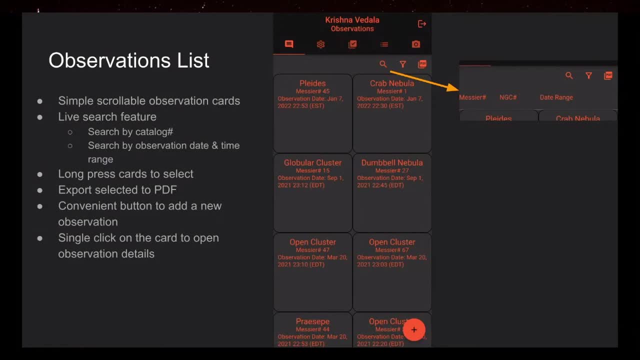 now, let's say i'm in a location where there's no internet, there's no cellular connectivity, there's no wi-fi. in that in in those situations, the data gets stored locally on the phone. that gets presented what and if you make any changes, those changes also get stored locally. 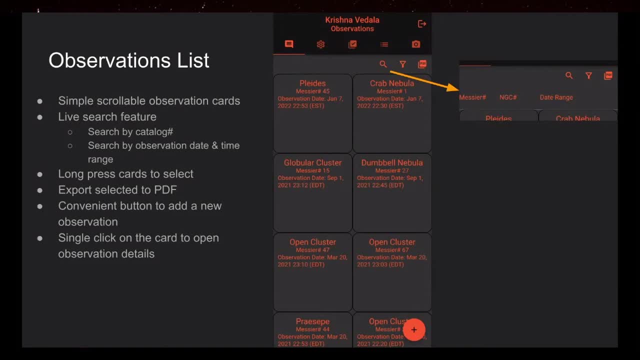 and once you have connection to the internet again, that would be updated automatically in the background. all that happens seamlessly without the end user getting affected or even being aware of it. now i'll just show a pouquinho on how i have pens on my phone, just in case i show clean again. you can get all of your information from me. 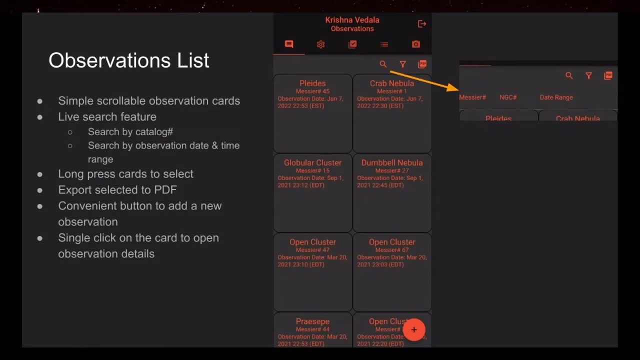 and then come plug it into any other roasting location here. so the uh return processing might be modified just by press check on the desktop. on the on the desktop you can see uh theme 1948. um sitio audio was updated to approximately five characters percent. even though you have things updating, it's not necessarily time saving. 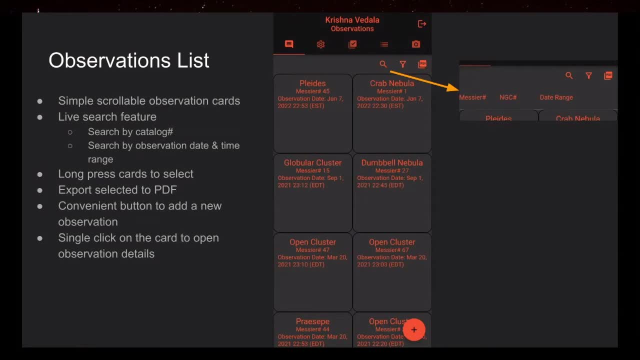 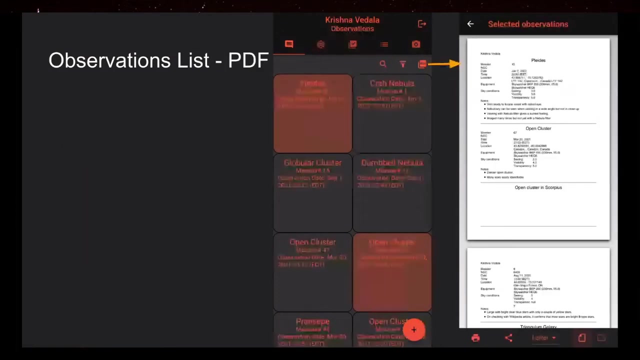 Once I have shortlisted the items, I can long press any of these tiles to select them, And when I click the PDF button on the top right, it would simply create a PDF page for me. like so, And this PDF file would have the name of the user. 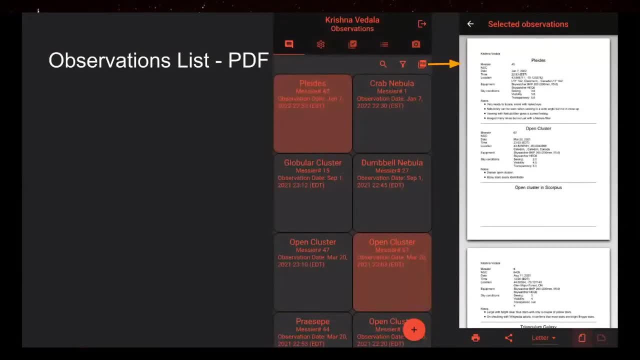 on the top left corner And, as a future add-on, I was thinking of adding a digital signature that would ensure and authenticate the PDF that was created, And this PDF you can then simply share with any user or, in fact, even RAC. 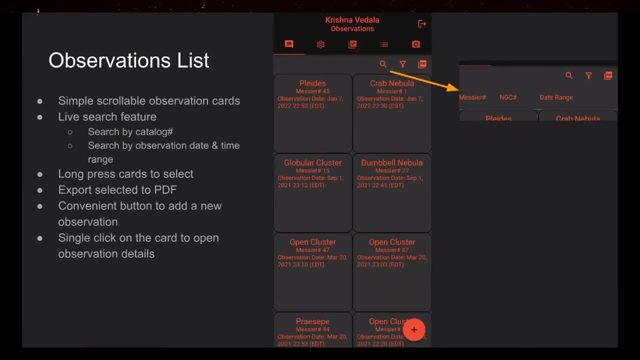 How can I record the observation? If you look on this observation page, on the top, on the bottom right corner, is a plus button. When you click that plus button you are led to record a new observation And in this, in this page, 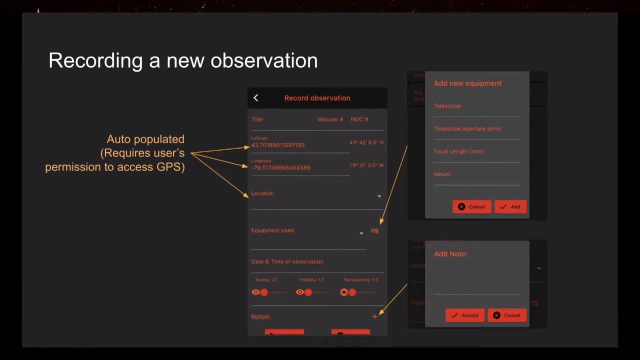 you're presented to enter title: the MSCA number, the NGC catalog number, if any, if you have to, but the title is important. The latitude and longitude values are acquired automatically if you authenticate the application to use your GPS location. 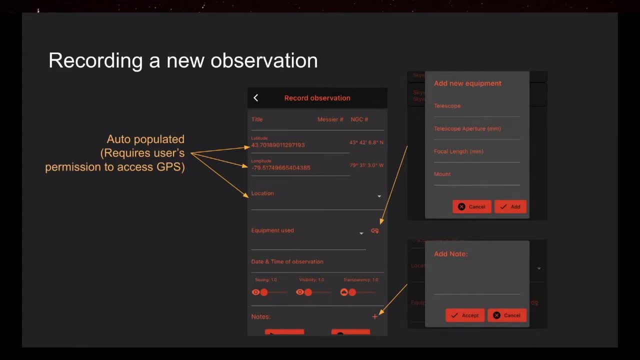 Similarly, the address location is also autofilled from on the Apple or Android devices. This tool is also available using a web interface, but on the web interface, some of this information you need to have to fill in manually, And so, while recording the observation, 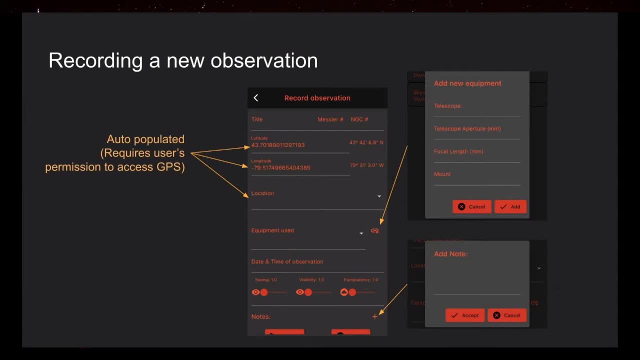 you can also mention which equipment was used, what were the seeing conditions, and you can add as many note points as you can to the list. It can be one 10.. You can edit, delete them today, tomorrow, anytime you want. 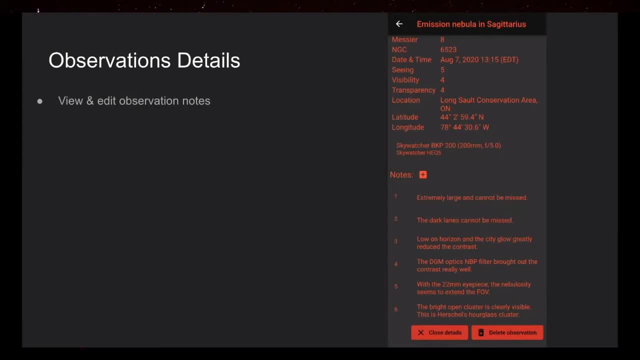 This is an example of one such observation that I made, where I have about six notes that I have done here. Swiping any of these notes can remove that particular note. You can add more notes later on, once you go back home and you think this is what I remember seeing. 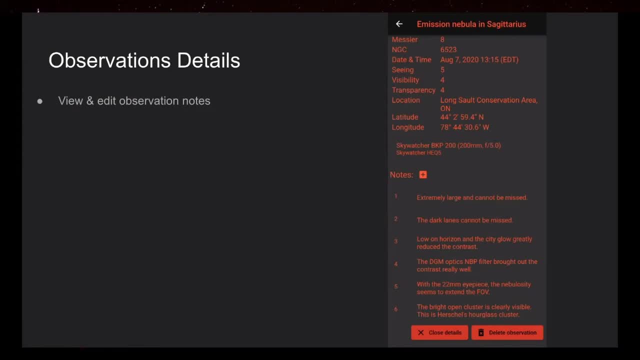 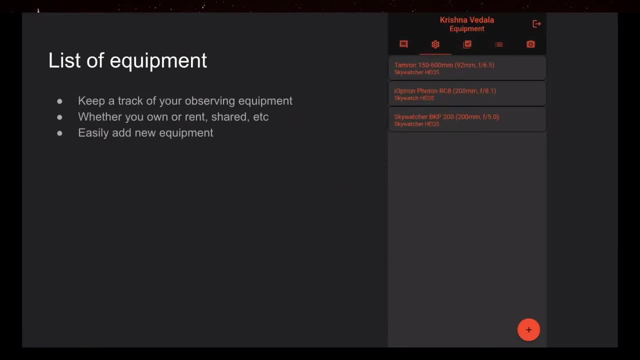 You can add that on later, And then you can add more notes in the list of equipment. As I said, today you might have an equipment consisting of an 18-inch telescope. Tomorrow you might upgrade it to a different 18-inch telescope. 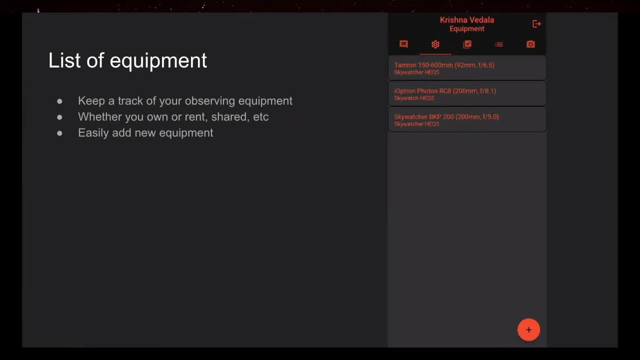 or even a 10-inch, or it might be that you went to DDO and observed using the BrickScope. In that case, you can absolutely add those information in here so that you can continue making your observations for posterity. one important thing that my wife and i thought of when we were, when we always go: 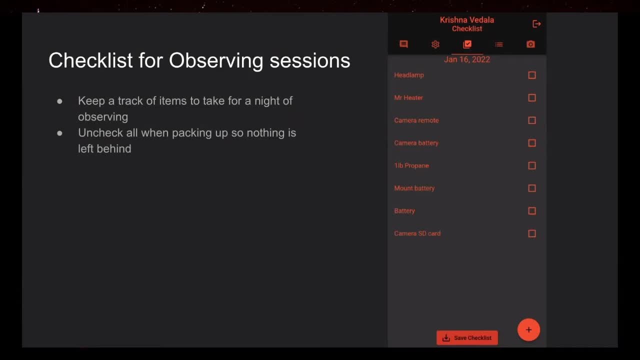 stargazing is the checklist of equipment that we want to take, and it has been numerous times that i forget one or the other, so i added a simple checklist of a checklist option where you can add your own items in there and every time you go, while packing up your equipment, you can check. 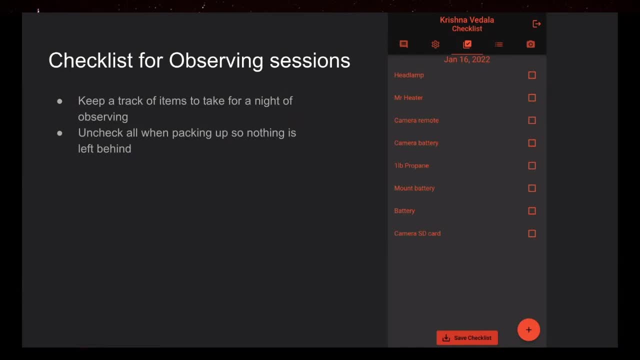 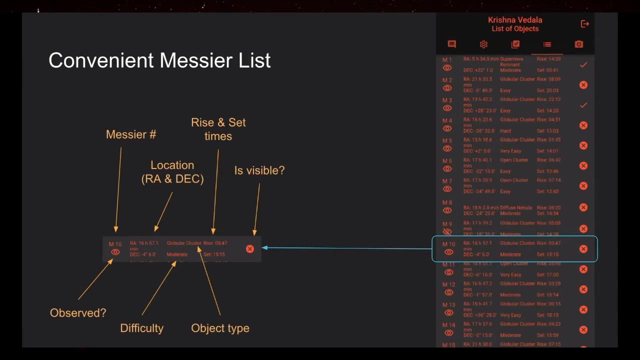 each box and once you're coming back, you can uncheck each of them in order to make sure whatever you took came back with you and you did not forget accidentally anything at the observing site. and this is the messy list that i added recently and that that was quite challenging. 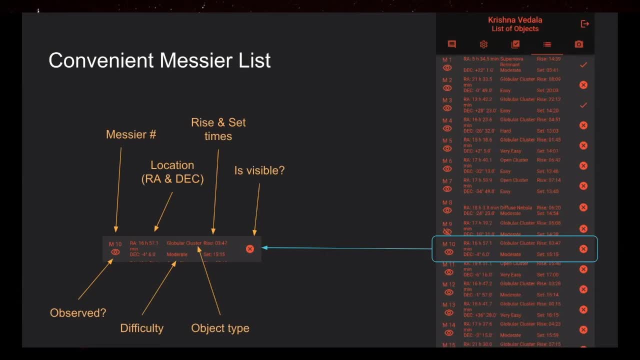 also fun to do. so this list- you can add your own items in there, and every time you go, while packing up your equipment, you can check each box. and every time you go while packing up your equipment, you can check each box- is a list of all the 110 messier objects. number one, two, um, each miss the the entire messier. 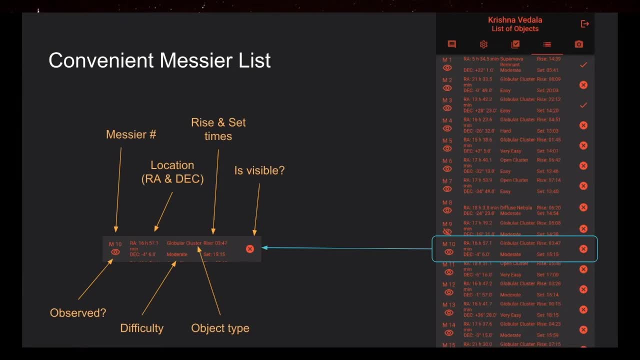 catalog was uploaded using an excel file to to a central database and that includes the um writer session and declination information for each of them and some some some information like what kind of a target it it is. is it a supernova remnant? it is a. is it a globular cluster? is it an open cluster? 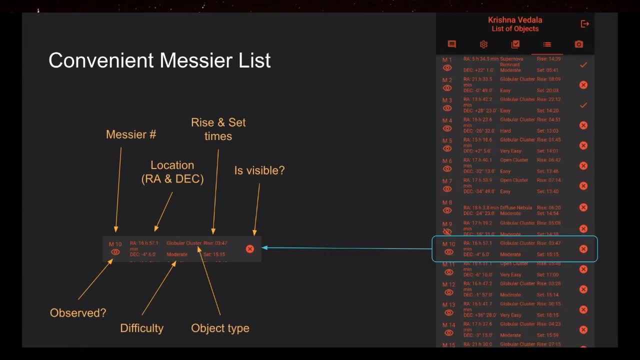 how easy or difficult is that target for us to observe? so, with re and declination and knowing the current location where the user is the cell phone, in fact, um, i went through and searched, come up with um, went through the um list of all the equations and came up with a simple structure. 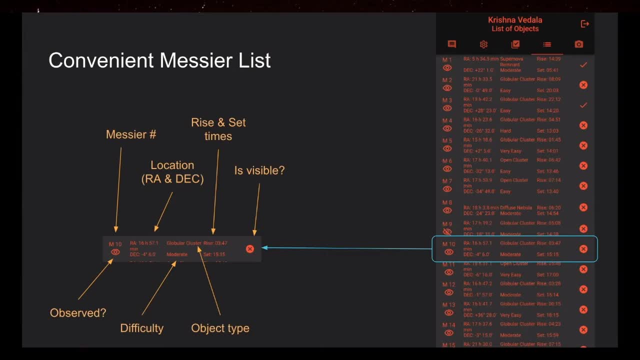 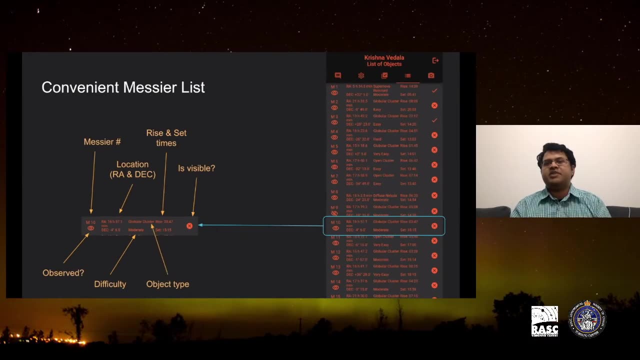 that can compute the rising time and setting time for each of these objects on the fly and present to you in this uh over here. because, as you know, based on your location, based on the time of the year, um, the rise and set times for these objects would change. 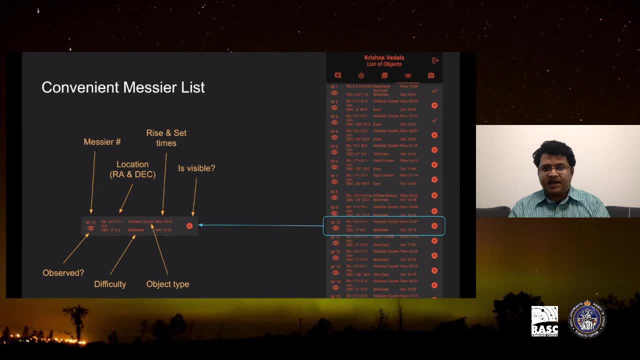 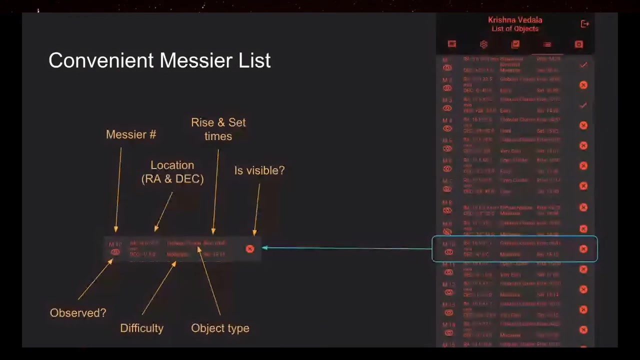 and, depending on that, you can. you can figure out which of these objects would be visible in the night sky tonight, um, and which of those would not be so. on the right hand side, the extreme right hand side, the x mark or the check mark indicates whether the 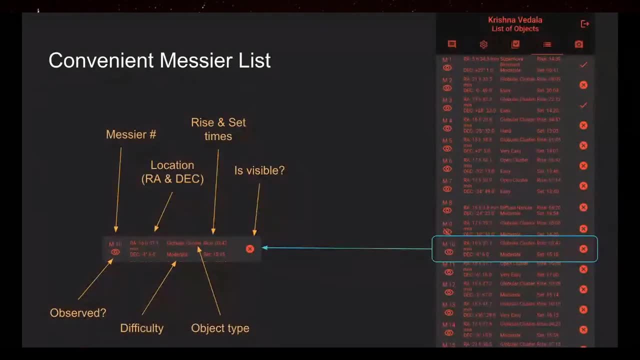 time window, the rise time and set time falls within the uh the night period and if it does, it gives you a checklist check mark that means you can go and observe it tonight. um, otherwise you see an x mark that means you cannot see it. um, it would not be so easy for you to watch uh in the night. 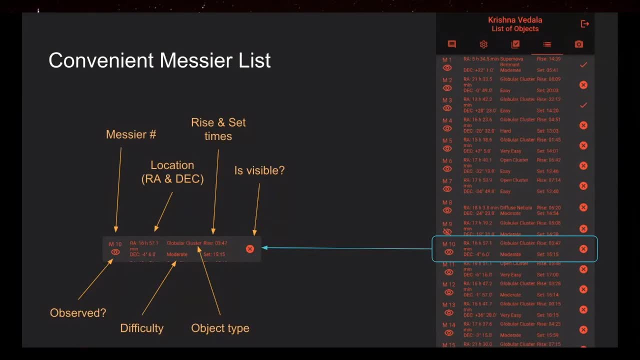 sky tonight, and um, and on the extreme left hand side. it also shows you which of these objects have i actually observed before. so, for example, m1, let me see one. i have a. i had observed it before and that's why it shows me that i symbol, whereas m9, um, is something that i haven't seen so far. 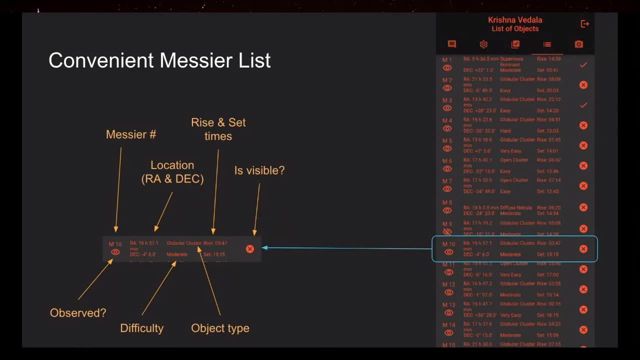 so it shows me that i symbol, with an oblique sign in front of it, um. so, in a, in a very convenient fashion i can, i can lower, i can um- go through the objects that i have not seen yet and which are visible tonight and check them off my bucket list. so i would be one step closer to achieving my certificate. 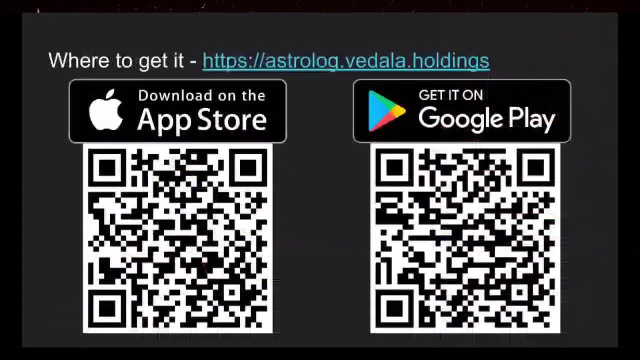 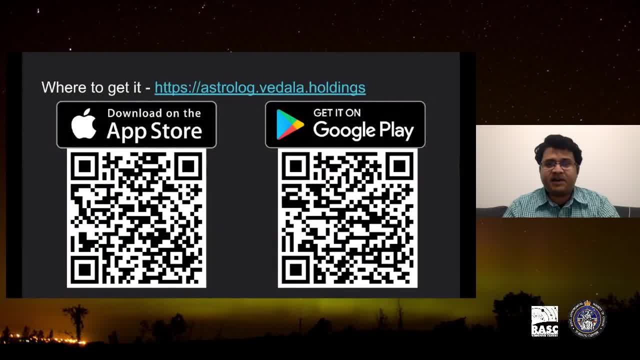 um, it was easy for me to build it over a couple of a couple of months and i initially built it for myself, um, and i thought if, uh, if people might find it useful, so i let it, um, uh, distribute. i just i distribute it for free, um, and you can download it on apple store and on google play. 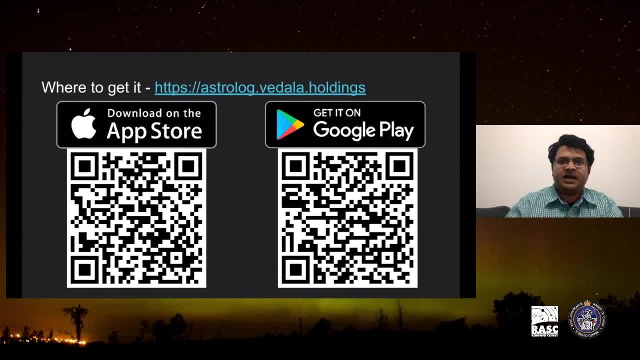 you can also try it on, uh, on the website up there: um, astrolog, Gospel, articlevirtual, longer настроlog, um, and also what i, uh, what i intended to do and i have done is that, um, i, i have released all the all the source code for this project for free on a repository system called GitHub. 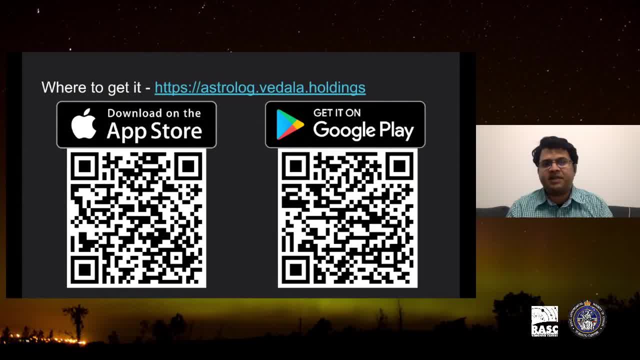 So if you're interested, feel free to let me know and I would be glad to share that information with you. Or if you actually search for Astrolog on GitHub, you should be able to find it. The code is pretty straightforward. It has been documented for everybody to use it. 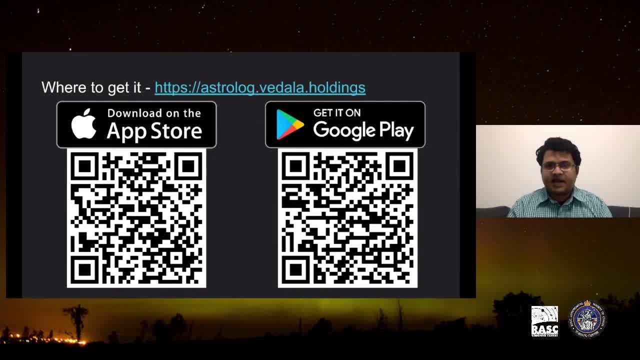 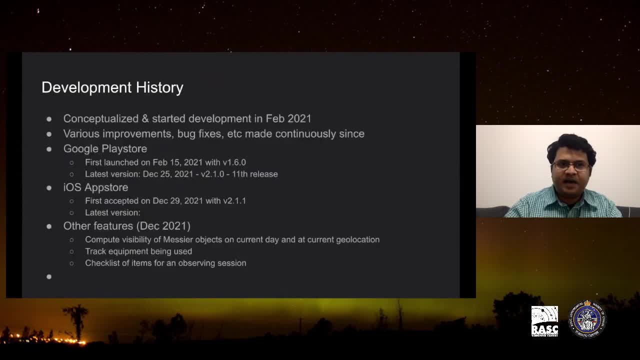 And if you are a programmer, you can absolutely create your own repository and develop your own app and install it for all your own use without having to rely on the backend infrastructure that I had set up. I initially conceptualized the project in February 21, and over a period of time slowly, 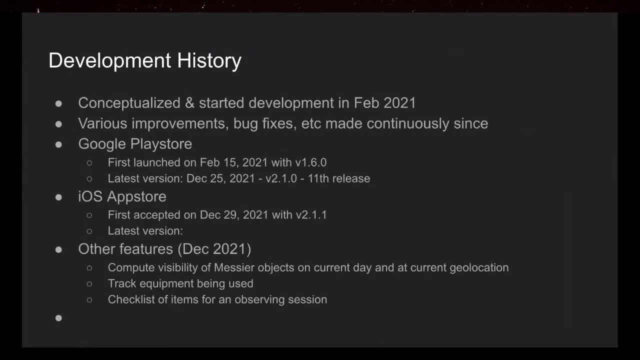 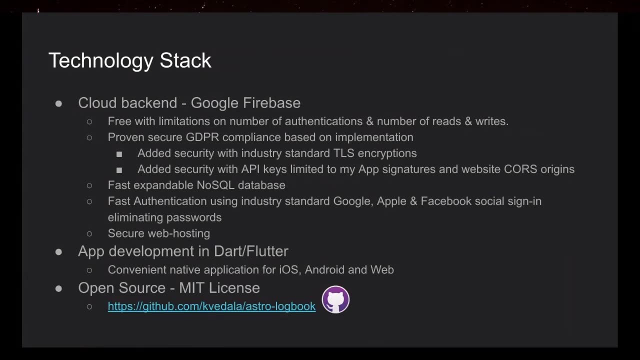 developed it, improved it and had a lot of fun using it myself. For whoever is technical in nature, this is the technology stack that I use. The backend uses Google Firebase. It is free for the application that I have, at least for myself. 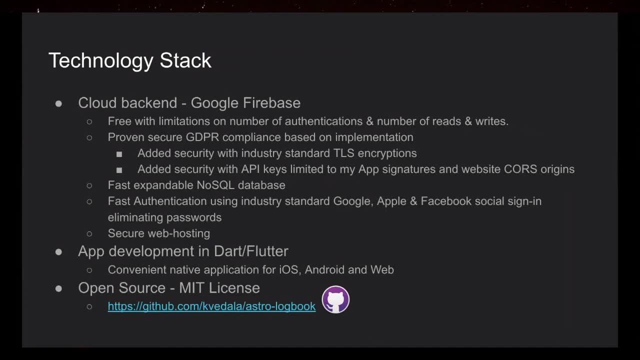 And even if many people start using it, it would still be free, unless it gets quite big, and then charges would kick in. But there are ways to get around that as well and it's quite easy to do, So I'm not too worried about it. 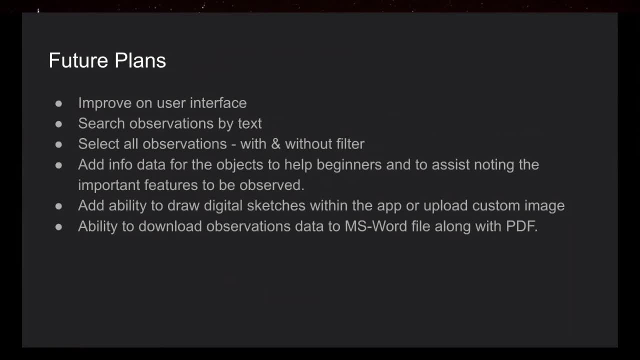 Future plans. So today I have the Macy catalog listed in. I want to add the NGC and the Caldewell as well. The user interface: it works for me but I'm pretty sure for various other people. we can adapt it and. 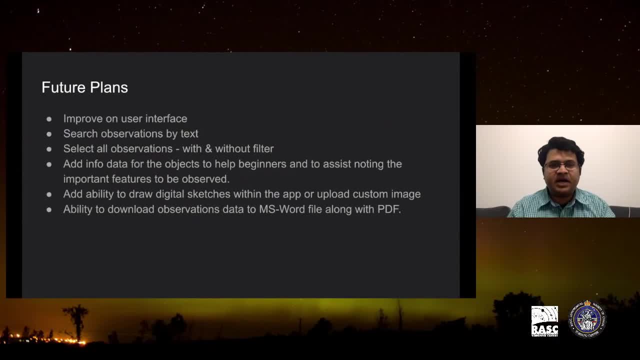 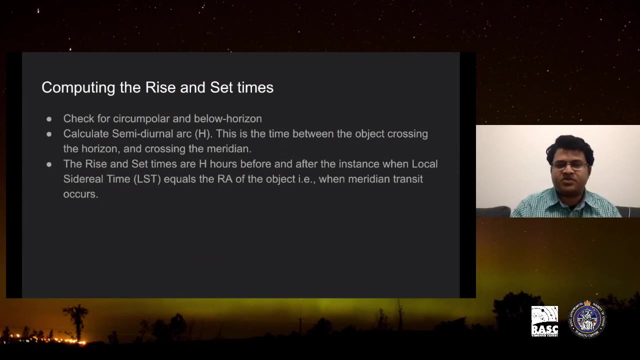 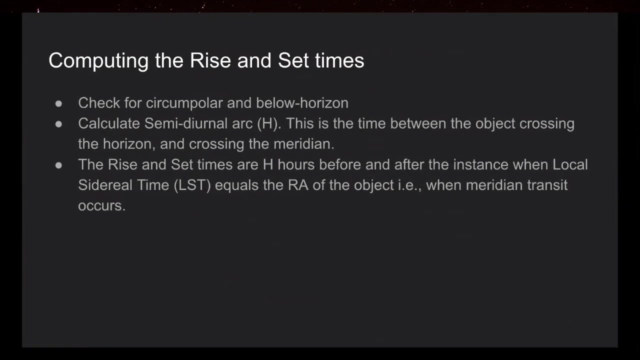 improvise on adding more features and more information to it. concisely, in a non-cluttered way. Computing the rise and set times was fun, like I said, and the equations? the funny thing with this was the equations were not clearly mentioned anywhere and there's no one location where I could go and say, hey, if I have RA, if I have declination information, latitude, longitude and the date time in UTC format. these are the steps to do so. 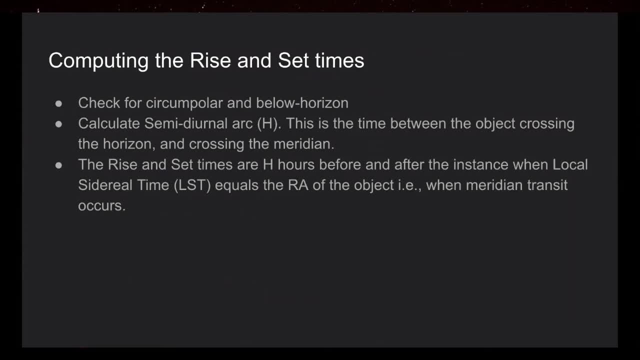 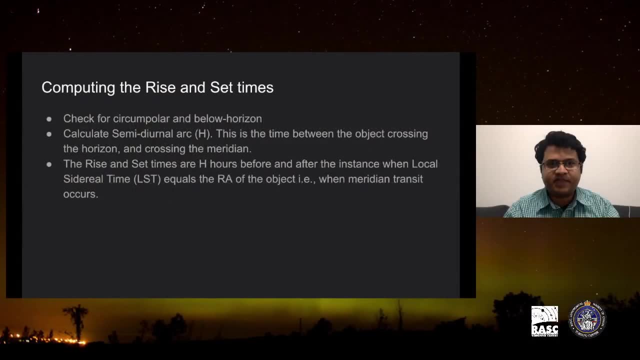 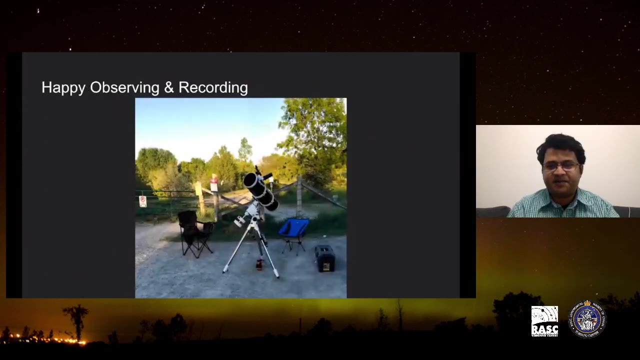 So that's why documentation. I documented all of that and I was going I would be uploading that information to the GitHub repository for people to be able to access it as well. So, given having said that, this has been very fun for me to do and to record my observations, I hope you guys find it useful as well. 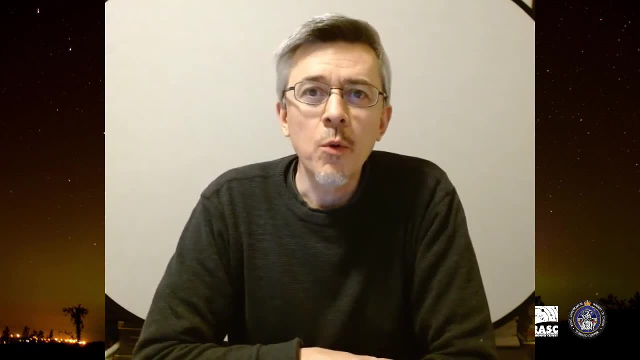 Thank you very much, Krishna, for sharing this with us and for the hard work and for, of course, sharing the source code for anybody who wants to use it. And if anybody's interested in doing a similar experiment, I'd love to hear what you think and how that would be. 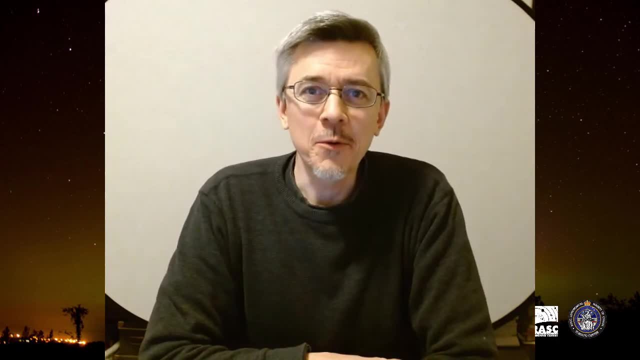 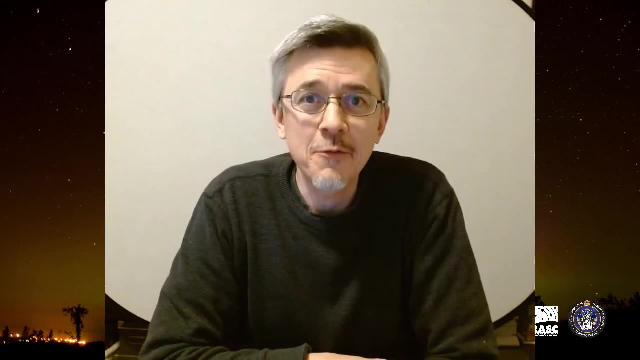 But also I understand people want to, you know, continue the development. That's fantastic. So we can see how capable our members are. It's quite something tonight, Lots of good stuff being shown. All right, Do we have any questions for Krishna Emma? 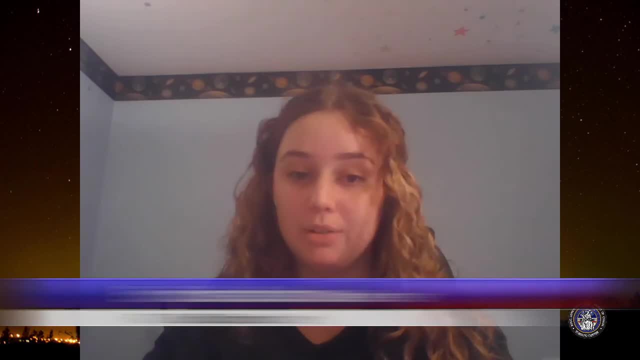 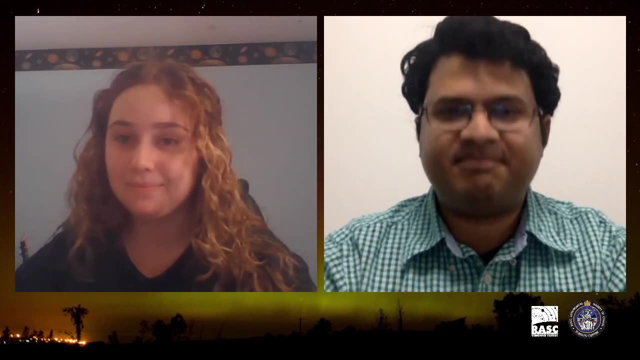 Yes, we have a couple of questions. The first one comes in from Ralph Chu. He says it looks like a great way to record observations for the Observance Pins programs. Thank you, That was lovely intention. i wanted to do it for myself and it just grew and thought it would be even. 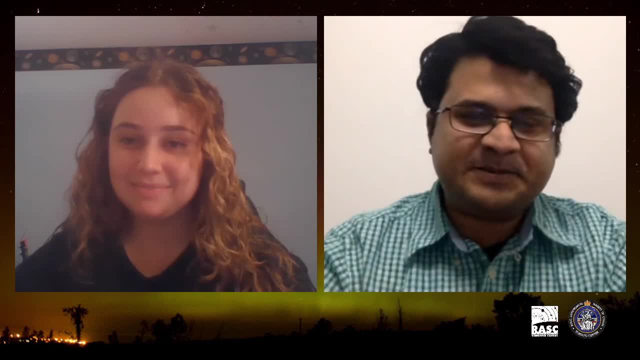 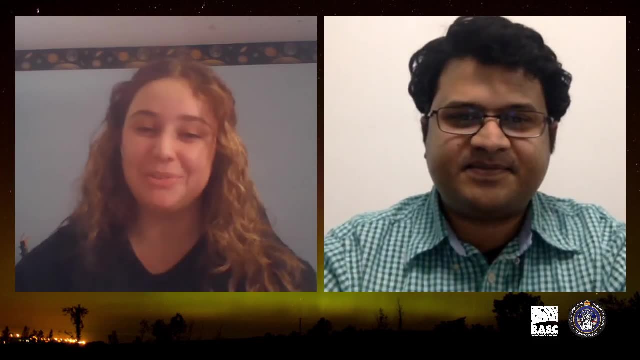 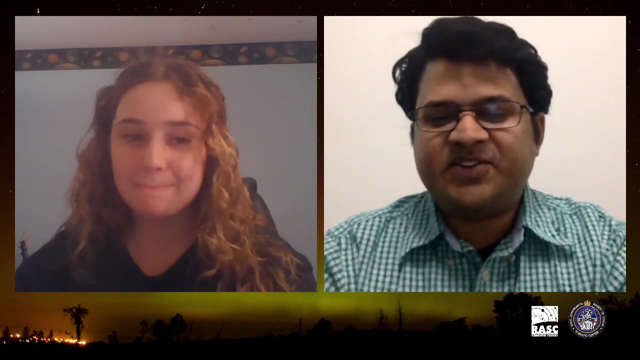 there's more scope to this than what i initially intended. cool, um, andy says for a future. sorry, andy wants to know for a future version. could we please get a place to enter variable star observations? absolutely so, um, in in the future. there is one. that's the next thing i wanted to. um, there are.